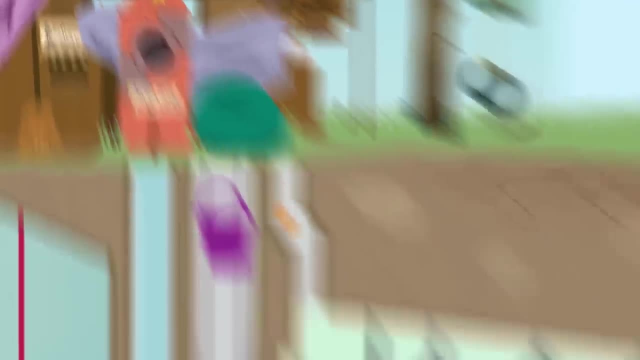 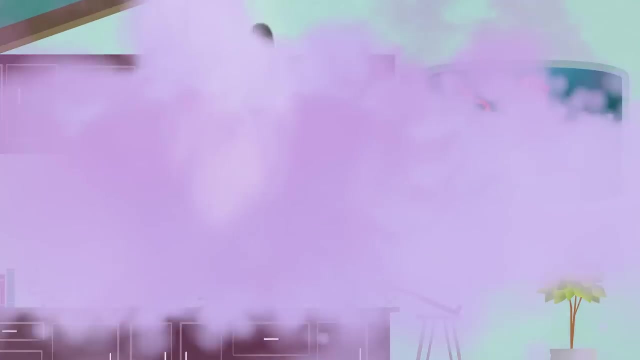 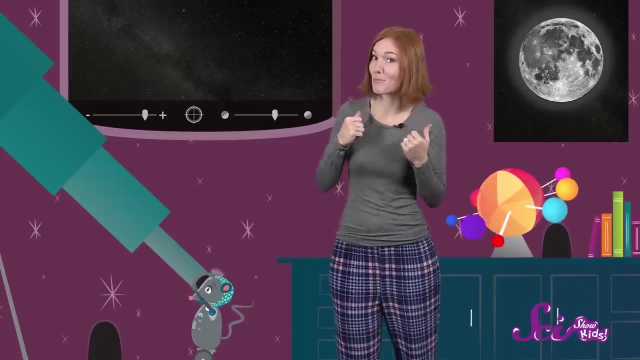 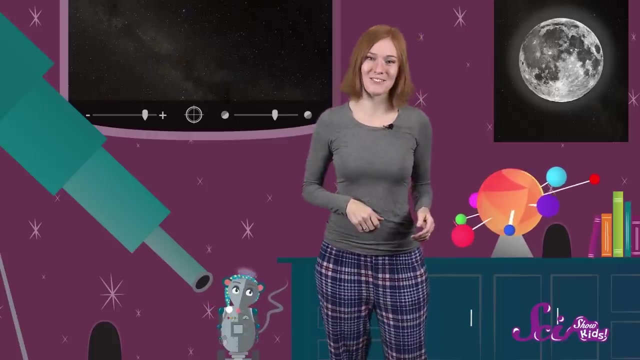 Oh, hey guys, It's just gotten dark here, so we're spending a little time before bed looking at the night sky, And sometimes we like to look up at the stars and make up funny stories about the things we see. Have you ever looked up at the clouds during the day and thought about what they looked? 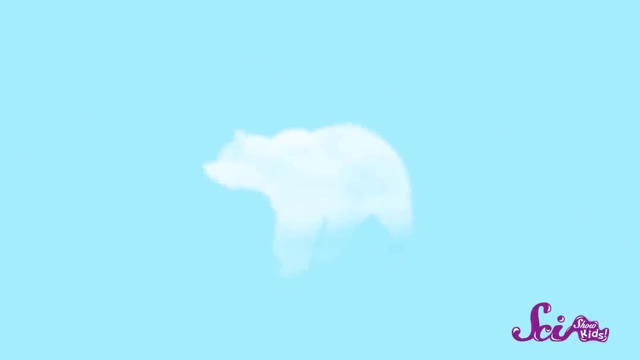 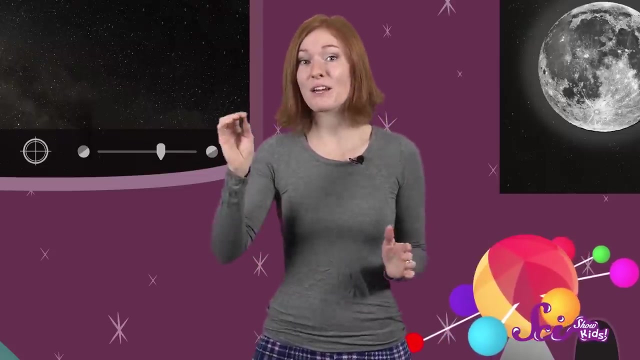 like A duck, an alligator, a shark or even a bear. Well, people do the same thing with the stars and they've done so for thousands of years. I'm sure you've noticed on a nice clear night how there are so many stars in the sky. 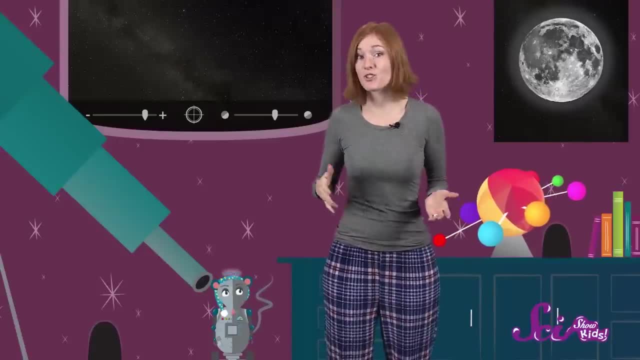 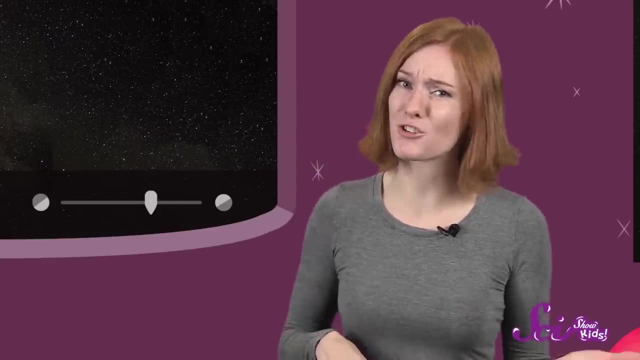 more than you can probably count. Some stars look brighter to us than others and the darker it is where you live, like if you're really far from the lights of a city, the more stars you can see And for a long time people have seen pictures among certain groups of stars, just like connect. 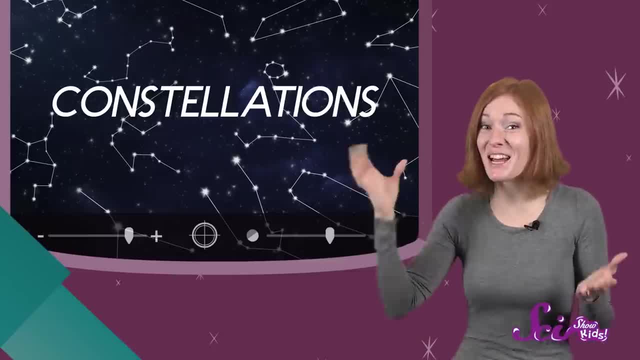 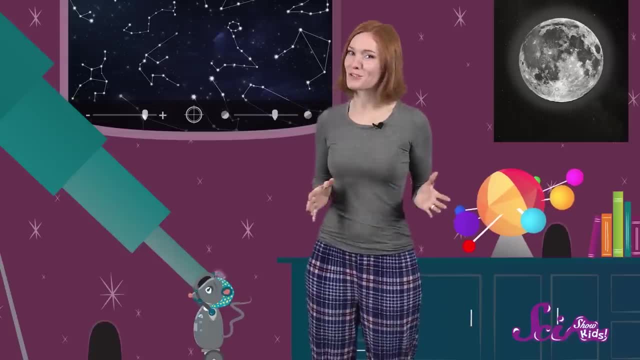 the dots. These groups of stars are sometimes called constellations, and scientists still use the names of these constellations to describe different parts of the night sky. Probably the most famous group of stars that's easiest to find is the Big Dipper, If you. 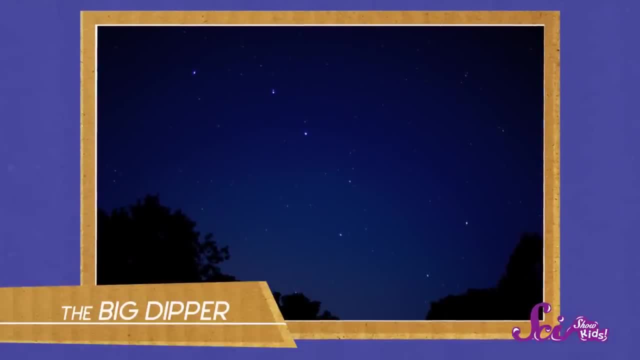 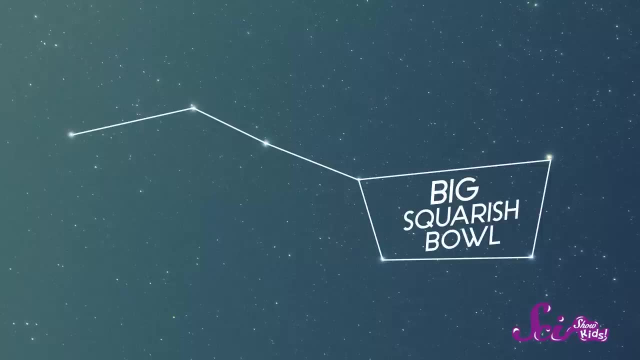 live in the Northern Hemisphere. you can spot it pretty easily in the northern part of the sky. It's made of seven bright stars and if you connect the dots of those stars you'll see a big squarish bowl with a really long handle sticking out of it. 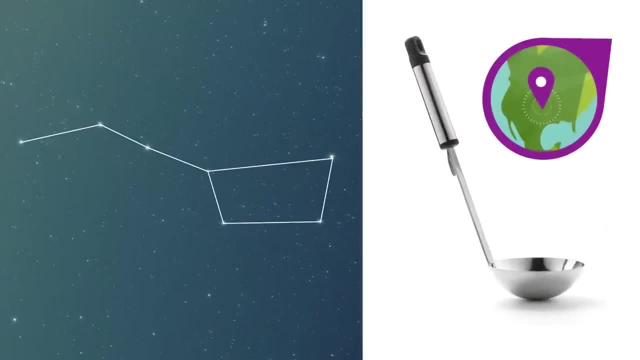 In the United States some people thought the stars looked like a big square bowl, but they're not. They thought the stars looked like a big ladle or spoon, so they called it the Big Dipper. But just like the fluffy clouds we were talking about, groups of stars can look different. 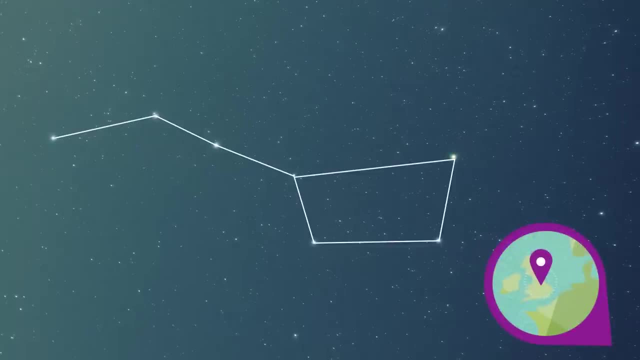 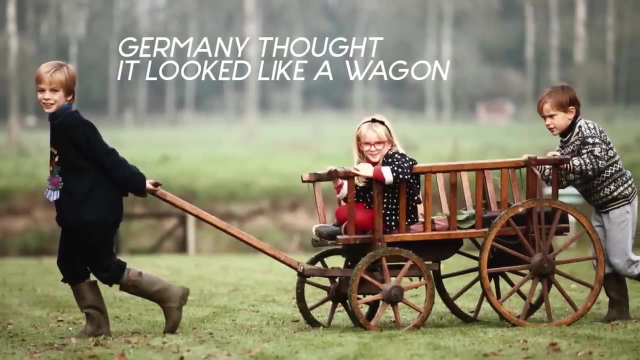 to different people. In Great Britain, for example, the same seven stars are called the plow because they were thought to look like a farmer's plow, And people in Germany thought it looked like a wagon. And those same stars also reminded lots of ancient people of a giant bear. 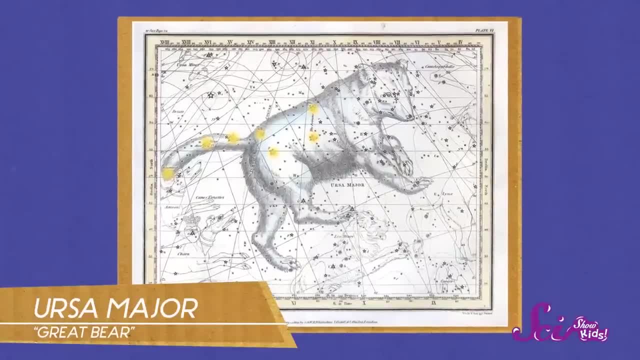 Scientists today consider the Big Dipper to be part of a bigger constellation that they call Ursa Major for Great Bear. The Big Dipper is easiest to find in the stars and it's the largest star in the world. You can find it in the summer when it's higher in the sky.